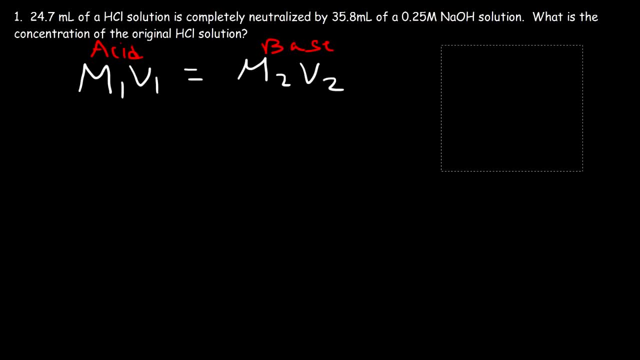 works for this type of problem. Okay, so in this example we're looking for the concentration of the original HDL solution. So looking for the concentration of the acid, M1V1 is twenty four point seven Milliliters. M two is point two, five moles per liter. V two is thirty five, And so we 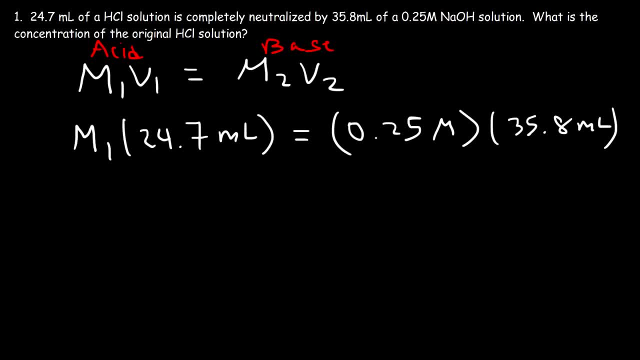 0.8 milliliters. So M1 is going to be 0.25 times 35.8 divided by 24.7.. So the concentration of HTL is 0.362 moles per liter, or simply capital M. 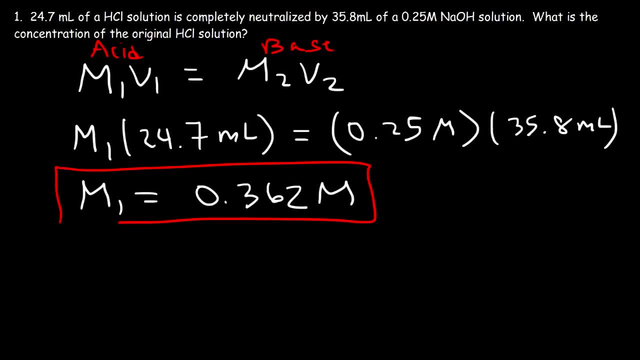 Now let's talk about the other method that we can use to get the same answer. This is probably the most simplest method to use, just using this formula if you have a monoprotic acid and base. Now to use the other method, you need to write a balanced chemical equation. 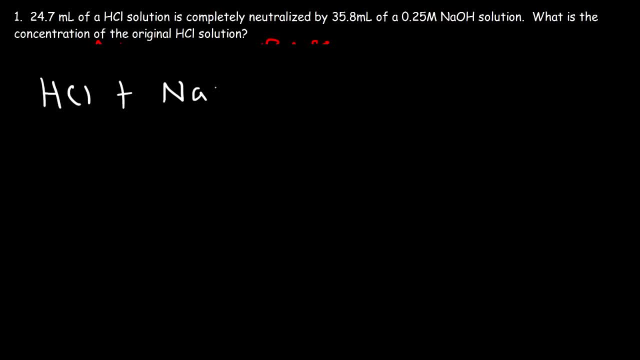 So HTL reacts with sodium hydroxide and HCl reacts with sodium hydroxide. So HTL reacts with sodium hydroxide and HCl reacts with sodium hydroxide and HCl reacts with sodium hydroxide. And this is a double replacement reaction. So H is going to pair up with OH producing. 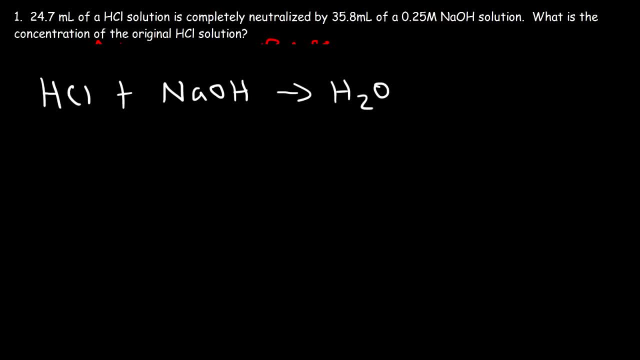 liquid water. And then Na is going to pair up with Cl, producing sodium chloride. So these two they react in a one-to-one ratio. The molar ratio is what we need in the balanced chemical equation. Now our goal is to find the concentration of HTL, So we need to start. 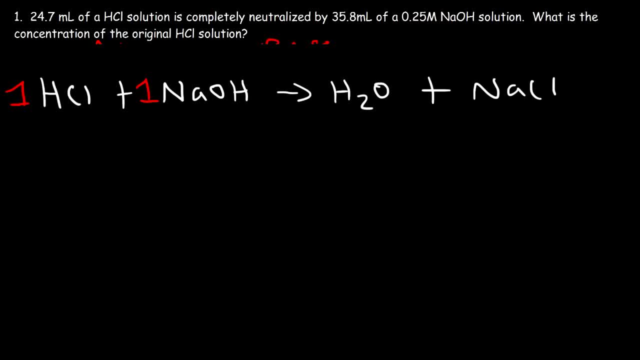 with the stuff of the other substance, Once we could find the moles of sodium hydroxide, the base that's going to equal the moles of the acid, And then, using the volume of the acid, we could find the concentration. So I'm going to start with the molarity of 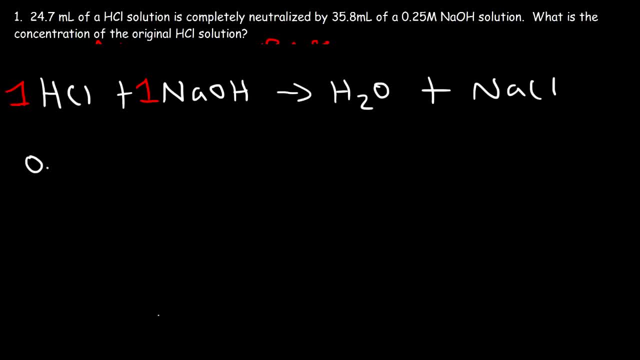 sodium hydroxide, But instead of writing as capital M, I'm going to represent it as moles per liter. So we have 0.25 moles of sodium hydroxide per liter of solution, And then let's multiply by the volume. To convert milliliters into liters we need to divide. 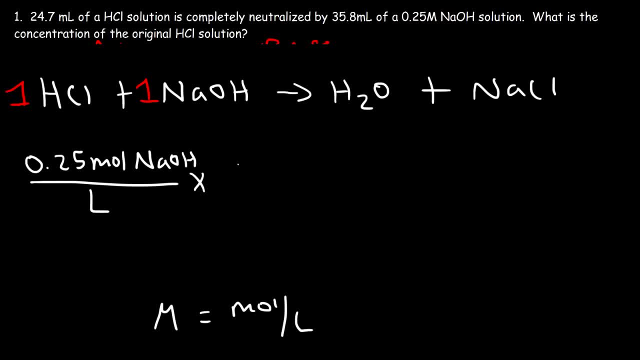 by 1000. So 35.8 milliliters is the same as 0.0358 liters. You can move the decimal point three units to the left. Now notice that the unit liters of solution cancels. So now we have moles of sodium hydroxide And we can convert it to moles of the acid using the. 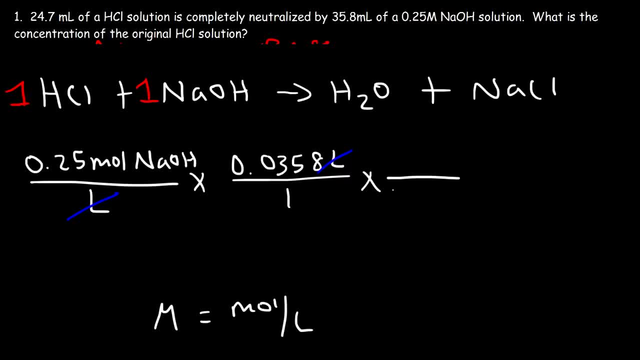 molar ratio which is one-to-one. So for every mole of NaOH that reacts, one mole of HDL reacts with it. So now the unit moles of NaOH cancels. So now we have moles of HDL. To get the molarity we need to divide. 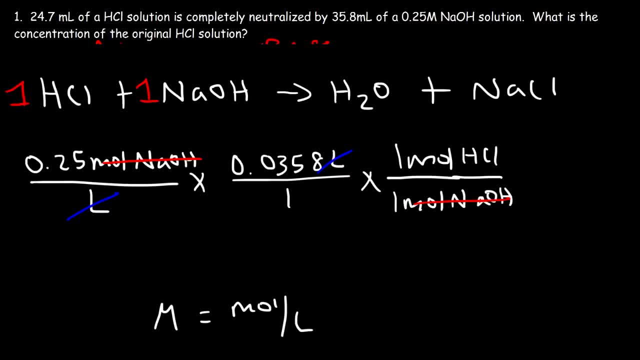 the moles by the liters And we have the volume of HDL. But we need to convert that to liters by dividing it by 1000.. So 24.7 milliliters is the same as 0.0358 liters. You can move the decimal point three. 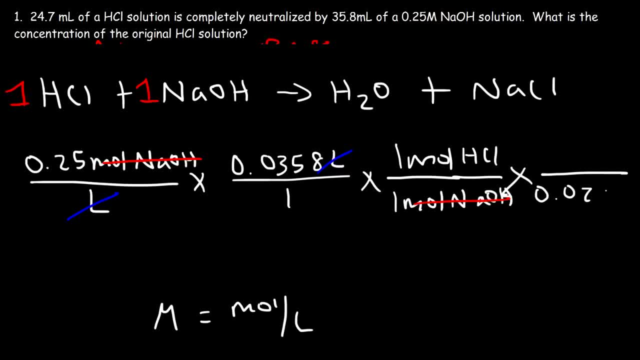 units to the left. So 35.7 milliliters is the same as 0.0247 liters. So to get the answer, it's 0.25 times 0.0358 divided by 0.0247. And you get the same answer: 0.362 moles per. 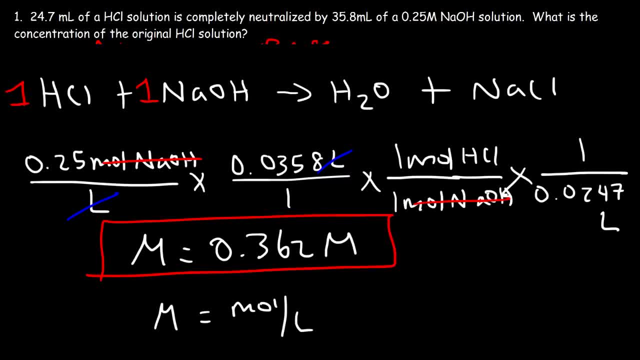 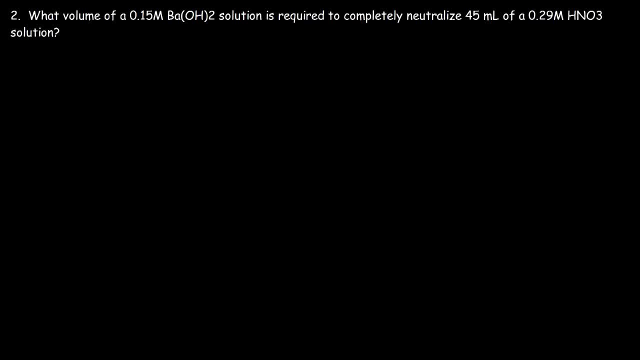 liter. So you can find the concentration of HDL using both techniques. Now, what about this one? So you can find the concentration of HDL using both techniques. Now what about this one? What volume of a 0.15 molar barium hydroxide solution is required to completely neutralize? 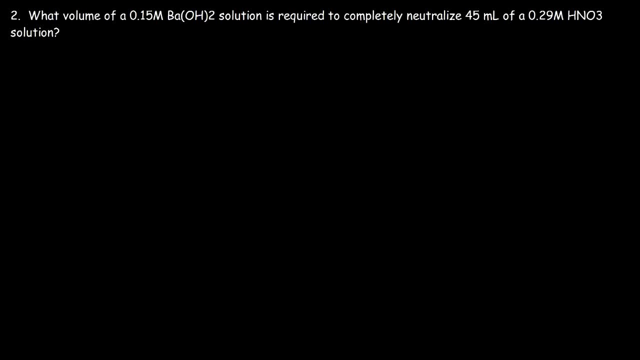 45 milliliters of a 0.29 molar HNO3 solution. So, like the other problem, we're going to get the answer for this problem using two techniques. So notice that nitric acid is monoprotic: It only has one hydrogen, But barium hydroxide has two hydroxides per formula. 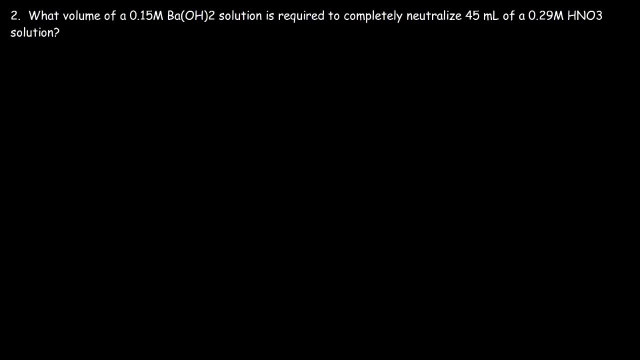 So, therefore, we need to modify the equation. So I'm going to write the acid first HNO3, and then the base, BAOH2.. Now keep in mind: the moles of the acid must equal the moles of the base in a neutralization reaction. 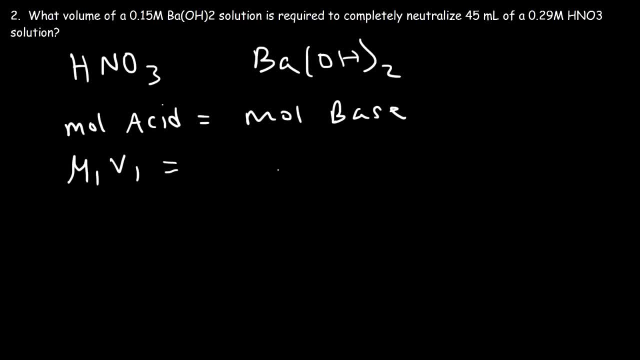 So M1V1,, which is the moles of the acid, equals M2V2, the moles of the base. But in this example barium hydroxide has two hydroxide ions per formula unit, So we need to incorporate that too. 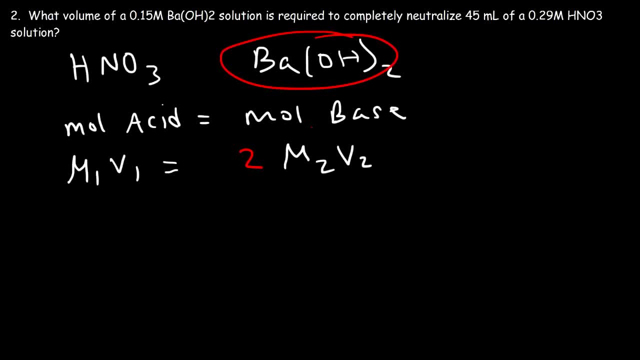 And we can put it on the same side that barium hydroxide exists. So M2V2 has to correspond to the base. We can only plug in the information of the base on this side. If we plug it in on the wrong side we're not going to get the right answer. 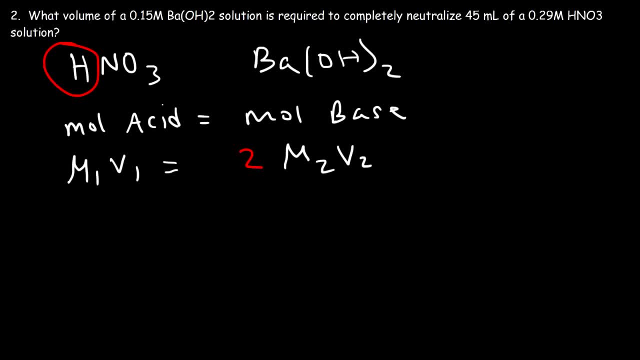 Nitric acid only has one hydrogen ion per formula unit, So We're going to put a 1 on the left side. Now let's go ahead and get the answer. So for the acid M1 is the concentration? It's 0.29.. 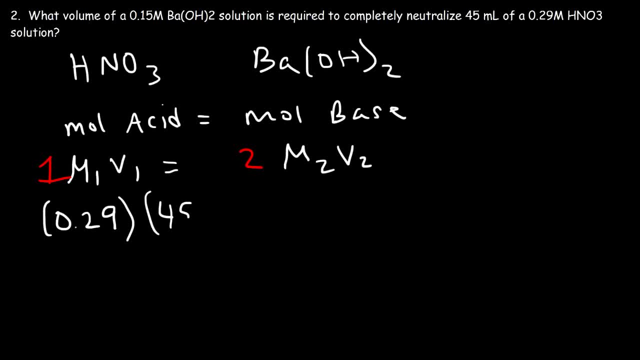 V1 is the volume: 45 milliliters. By the way, if V1 is in milliliters, V2 has to be in the same unit, milliliters. If V1 is in liters, V2 has to be in liters. 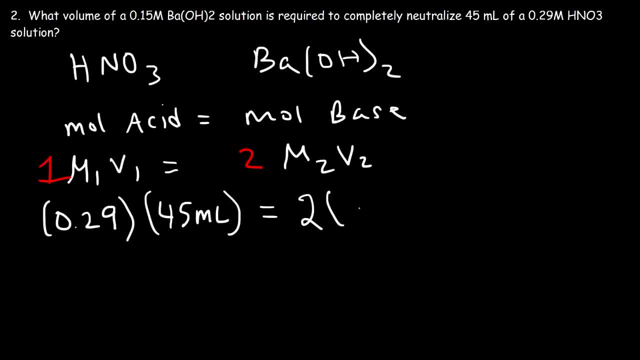 The unit has to match. Then we have a 2. in front, We have the molarity of the barium hydroxide solution, That's 0.15.. All we need to find is V2.. So now we just got to do some math. 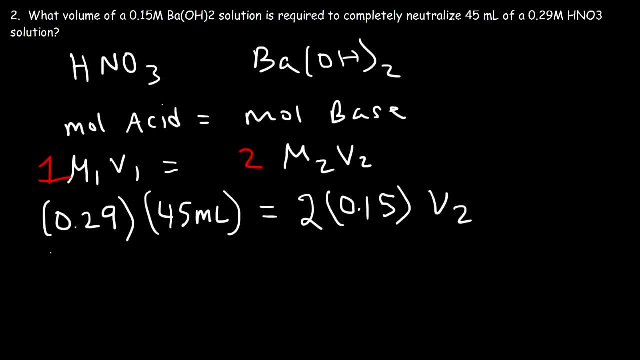 0.29 times 45 is 13.05.. 2 times 0.15 is 0.30.. So to find V2, all we need to do is take 13.05 and divide it by 0.3.. 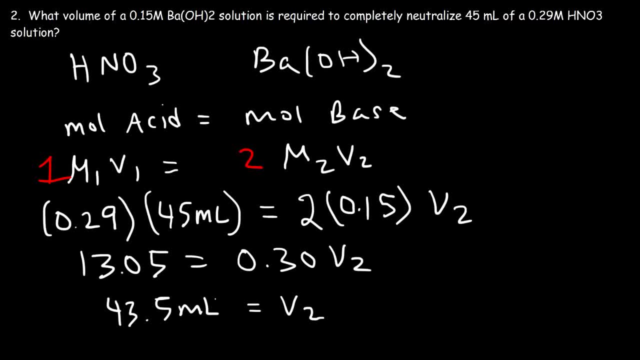 So V2 is 43.5 milliliters, So we have to find V2.. So that's the answer to the problem, which I'm going to rewrite it here for reference. So let's see if we can get the same answer using stoichiometry. 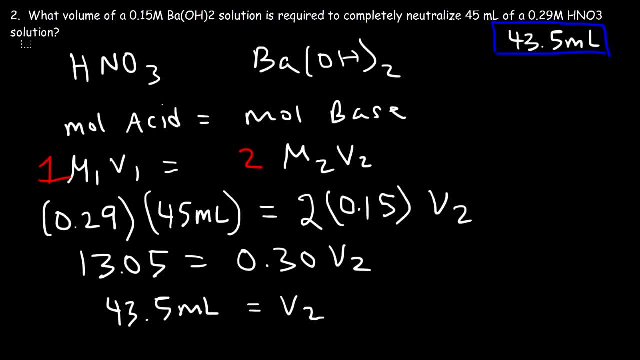 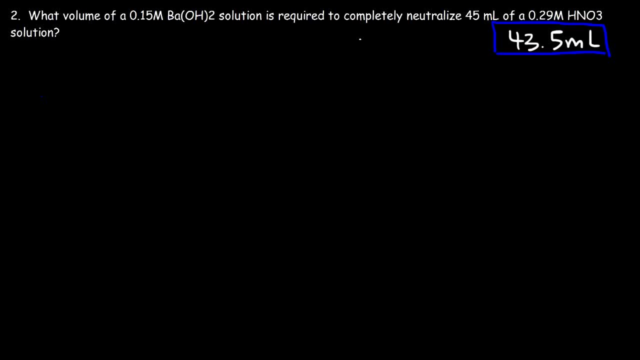 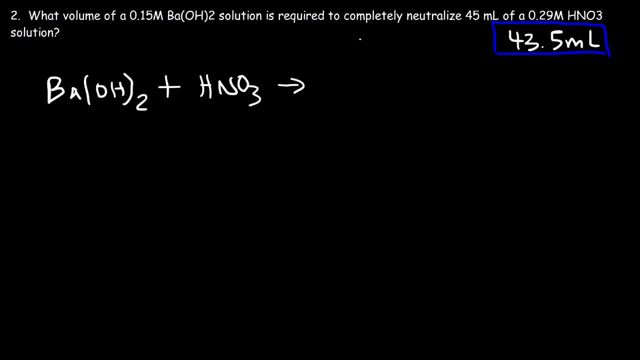 0.25 reacts with 0.25.. 0.25 reacts with 0.25.. Now, when H and OH get together, it's going to produce water, as always. Now, what about when barium pairs up with nitrate? 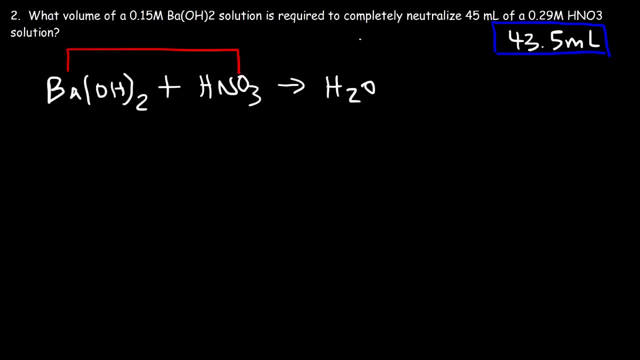 What's the chemical formula between those two ions? Barium has a positive 2 charge. It's in group 2 of the periodic table. plus, it has two hydroxide ions attached to it, And you know each hydroxide ion has a charge of negative 2.. 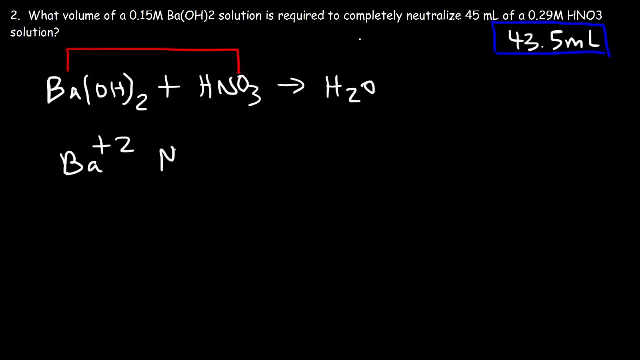 negative 1, so barium has to be plus 2.. Nitrate has a negative 1 charge, so the chemical formula for barium nitrate is Ba1 and O3, 2. Now we need to balance it. We have two nitrate ions on the right side, so we 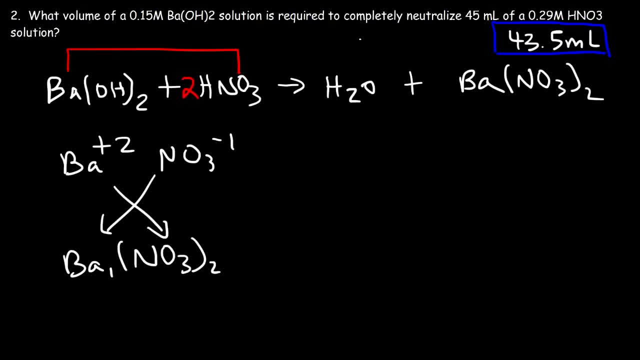 need a 2 in front of HNO3. And we have two hydrogens here, two hydrogens there, so there's a total of four hydrogens on the left. so we need to put a 2 in front of water so we can have four hydrogen atoms on the right. So now the chemical. 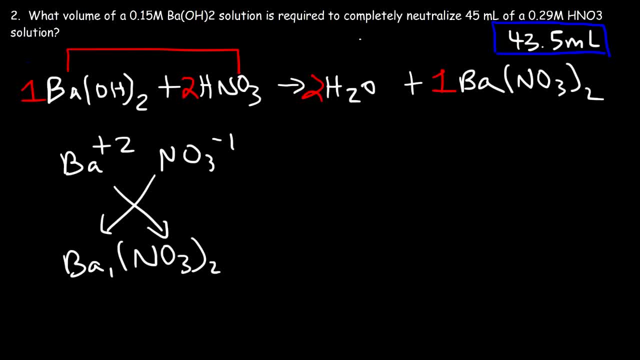 equation is balanced, but what's important is the molar ratio between barium hydroxide and nitric acid. It's a 1 to 2 ratio. That's why we need to write the balanced chemical equation to get that molar ratio. So now let's go ahead. 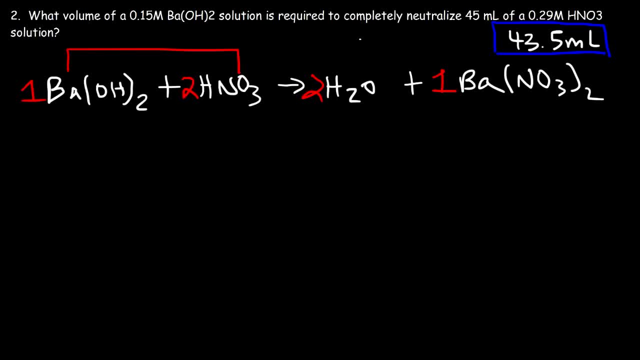 and calculate the volume of barium hydroxide. So let's start with the other substance, nitric acid. Let's get the moles of the acid first. So instead of writing 0.29m, I'm going to write 0.29 moles of nitric. 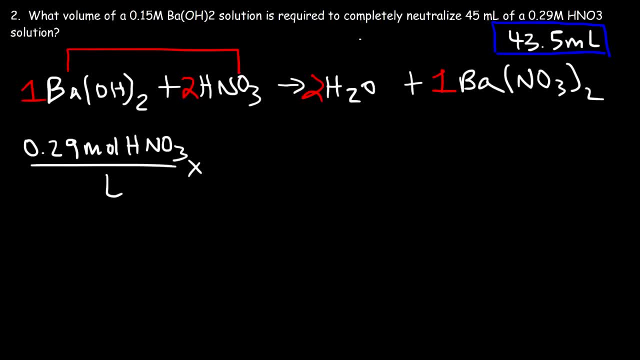 acid per liter of solution. Next, let's multiply by the volume of nitric acid, So we have 45 milliliters, and if we divide that by a thousand, that's 0.045 liters. So now we have the moles of the acid. 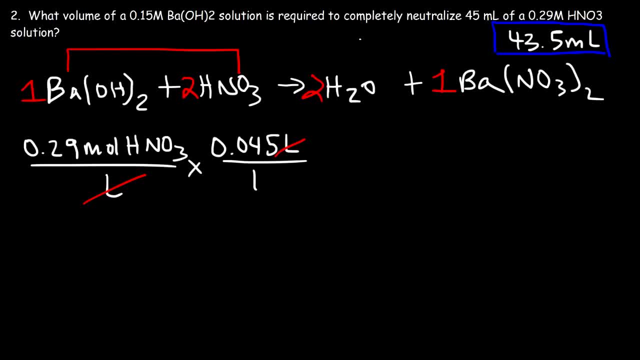 Now let's convert it to the moles of the base using the molar ratio. So for every two moles of nitric acid that participates in a reaction, one mole of barium hydroxide will react with it. So now we can get rid of the unit moles of nitric acid. Now the last thing we need is: 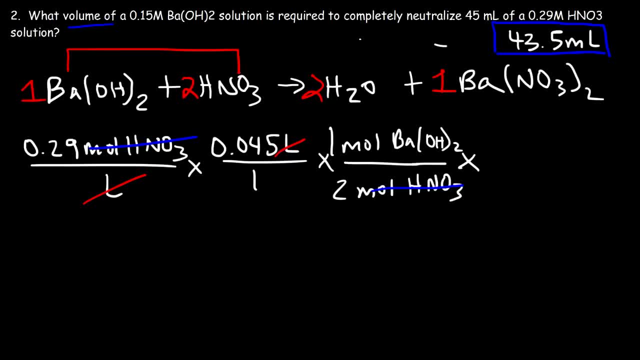 the volume. Let's get the volume in milliliters. Now we have the concentration of barium hydroxide. The molarity connects moles and liters together. So a 0.15 molar solution means that there's 0.15 moles of solute per one liter of solution. So 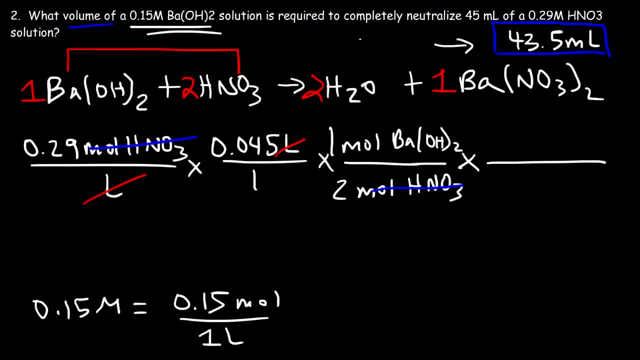 since we have moles of barium hydroxide on the top, we need to put moles of barium hydroxide on the bottom. So one liter of barium hydroxide solution contains 0.15 moles of BaOH2.. And I'm running out of space here, So we can cancel these two. 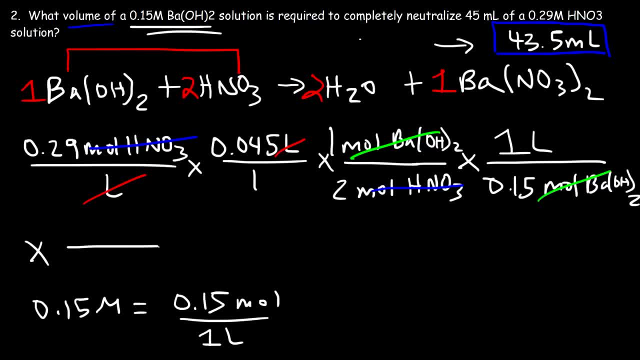 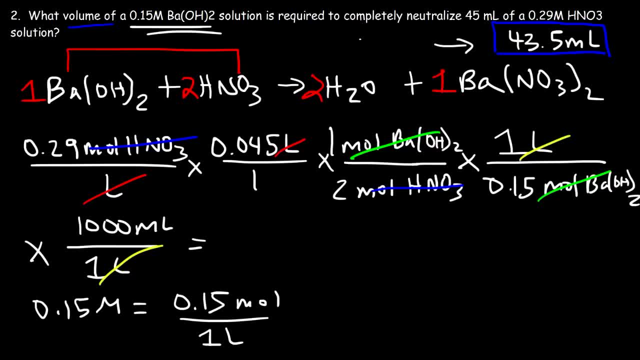 So it's 0.25 times 0.45, divided by 2, and then take that result divided by 0.15, and then multiply it by a thousand, And this will give you the same answer: forty three point five milliliters. 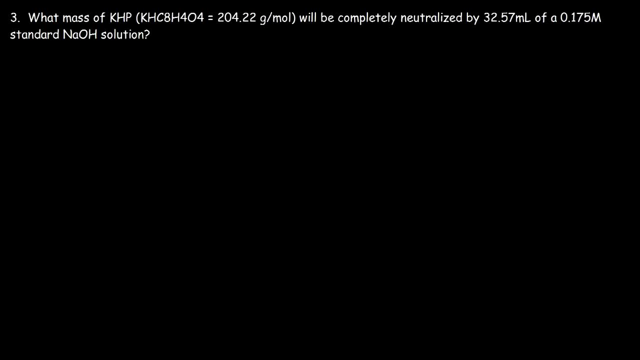 Number three: what mass of KHP? potassium hydrogen phthalate will be completely neutralized by 32.57 of a 0.175 molar standard sodium hydroxide solution. so what do you think we need to do in this problem? need to understand that KHP is a mono. 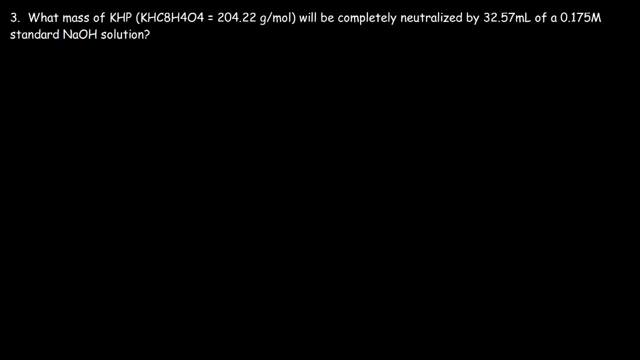 aprotic acid, and we can't use the formula m1- v1 equals m2- v2, because that formula doesn't correspond to mass. so the best way to get the answer is by stoichiometry. this might be bad news for those of you who really like those formulas, but let's start with a balanced chemical. 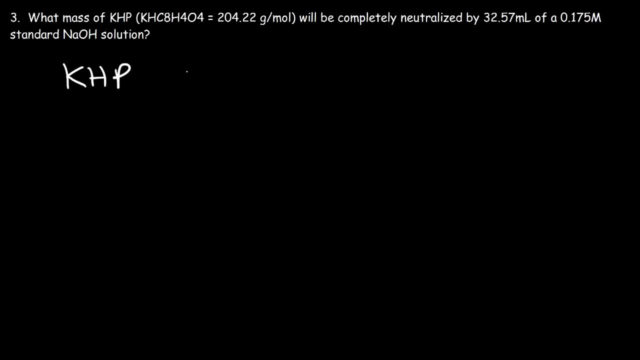 equation. so KHP reacts with sodium hydroxide. if you want to, you can use this, but I'm just going to use KHP. what you need to understand is that this hydrogen will combine with the hydroxide ion produced in water and once you take 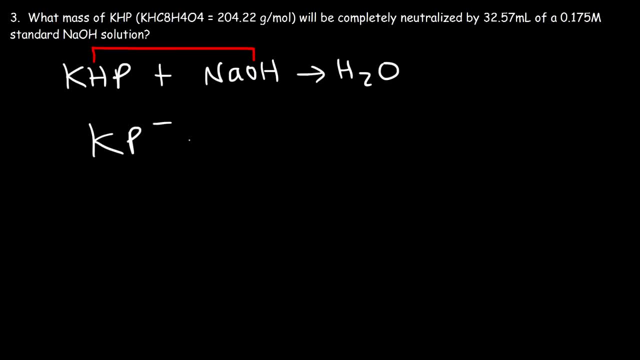 away the hydrogen, what's left over will have a negative charge and that's going to cause a negative charge and that's going to cause a negative charge and that's going to pair up with the sodium. so this is going to be and a K P. if you want to, you can replace the P part with c8 h4o4. I'm gonna write as: 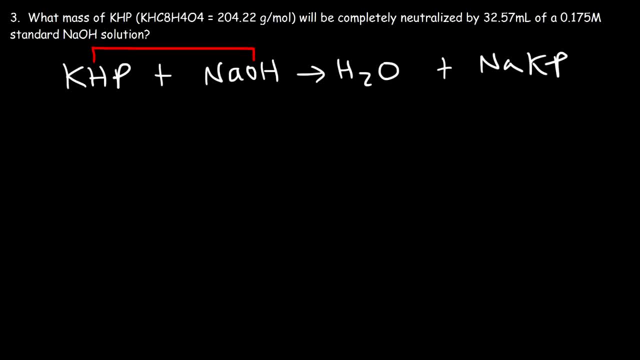 KHP, because it's a lot simpler. so now notice that in a balanced chemical reaction, KHP reacts with sodium hydroxide in a 1 to 1 molar ratio, and that's what we need. as you can see, there's only one acidic hydrogen in KHP. the other hydrogen's are: 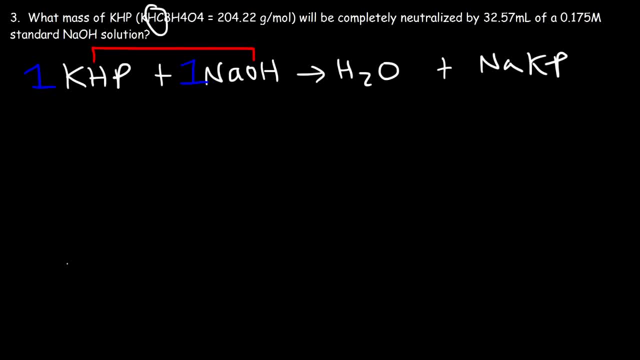 not acidic. only the one that's lifted, excuse me, listed to the left is the one that's acidic. so what we're going to do is start with the information of certain hydroxide. we can get the moles of any oh, then use that to get the moles of khp and 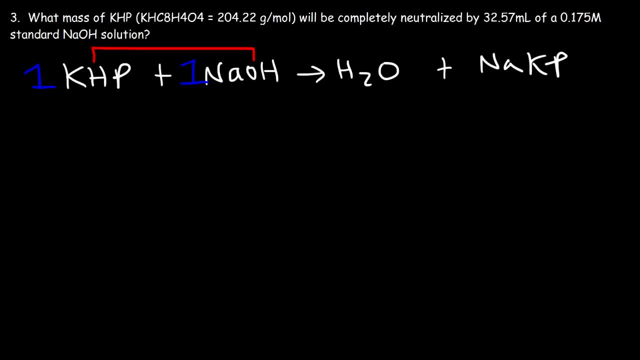 then use the molar mass of khp to get the grams. so if you understand how to do it, feel free to subscribe to our channel to pause the video and try, If not, sit back and watch. Let's start with 0.175. 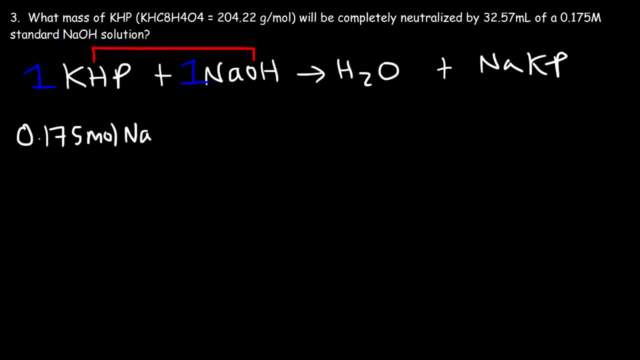 moles of NaOH per liter, as we've been doing before, And let's multiply that by the volume of the NaOH solution. but we need this in liters. So if we divide that by thousand that's going to be .0357 liters. Now let's 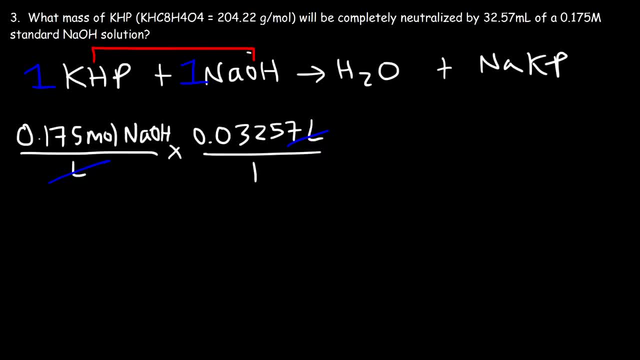 convert from moles of NaOH to moles of KHP, so it's a 1 to 1 ratio. For every mole of sodium hydroxide that reacts, one mole of KHP will react as well. Now the last thing we need to do is we need to. 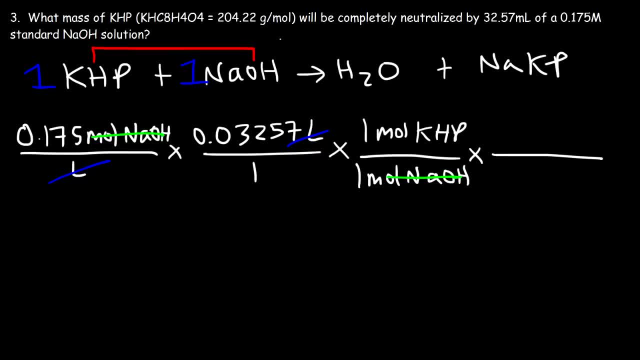 convert the moles of KHP into grams using the molar mass. So one mole of KHP has a mass of 204.22 grams, And so now all we gotta do is just get the answer. So let's multiply 0.175 by 0.03257 and then multiply that result by 204.22.. 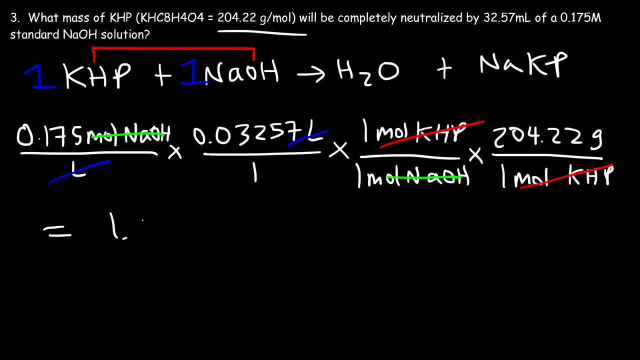 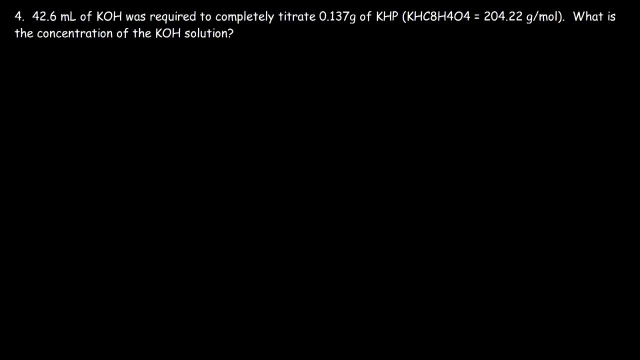 So the mass is equal to 1.164 grams of KHP. So this is the answer Number 4.. 42.6 milliliters of KOH was required to completely titrate 0.137 grams of KHP. What is the concentration of the KOH solution? 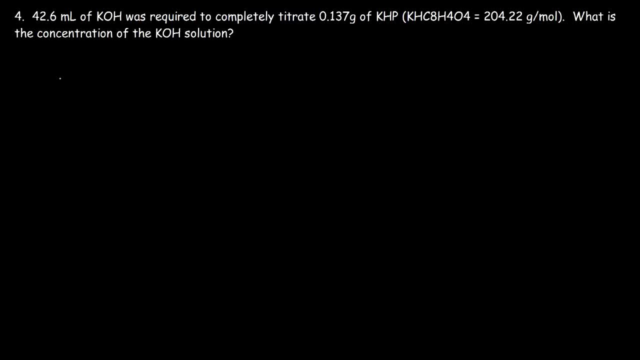 0.137 grams of KOH was required to completely titrate 0.137 grams of KHP. What is the concentration of the KOH solution? What is the concentration of the KOH solution? Well, let's begin. So. KHP is going to react with KOH And every time H and OH gets together. 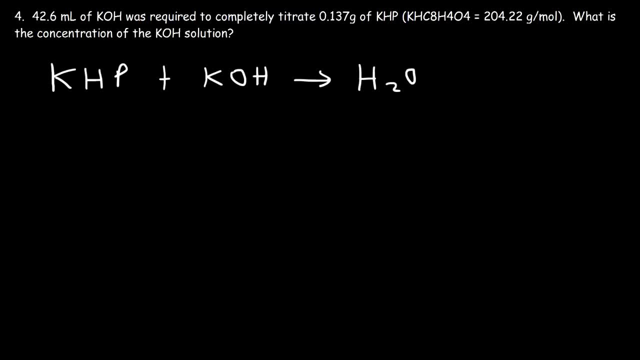 they're going to produce water. After that we're going to combine K with KP. So that's going to be K2P, And keep in mind P is C8H4.. So that's going to be K2P And keep in mind P is C8H4. 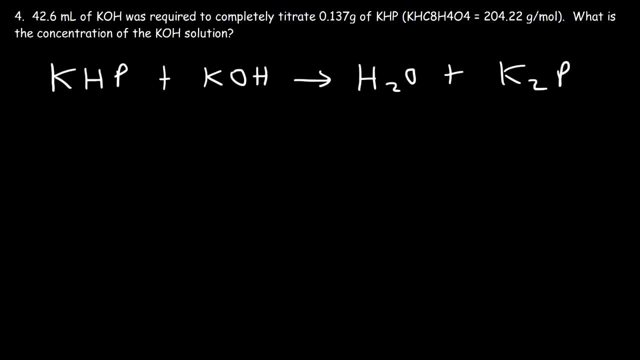 So, once again, we have a one-to-one molar ratio, which is what we're looking for in this example. So, once again, we have a one-to-one molar ratio, which is what we're looking for in this example. So we want to find the concentration of KOH. Therefore, start with the other substance, KHP.